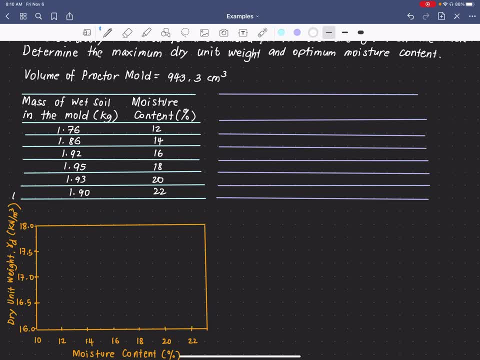 And the dry unit weight should be in kilonewton per cubic meter, And the given data is the mass of wet soil in kilograms. The volume is given, and so we can compute for the unit weight. We need to solve for the moist unit weight first and then calculate the dry unit weight for each. 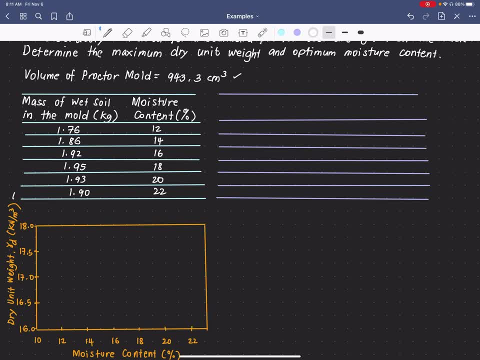 And then we can calculate the mass of wet soil in kilograms. So I have prepared another table here for us to calculate the wet unit weight or the moist unit weight of soil. So to do that, let us convert first the mass of wet soil into the weight of wet soil. 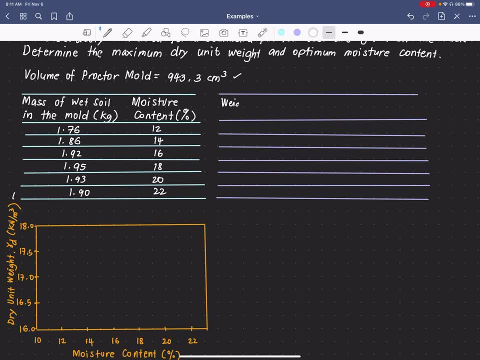 Let us write: This is in kilogram, So we need the weight, So let us have it in newton. Then, after solving for the weight, we can calculate now the moist unit weight using our formula, And that is our gamma, And the unit here should be in kilonewton per cubic meter. 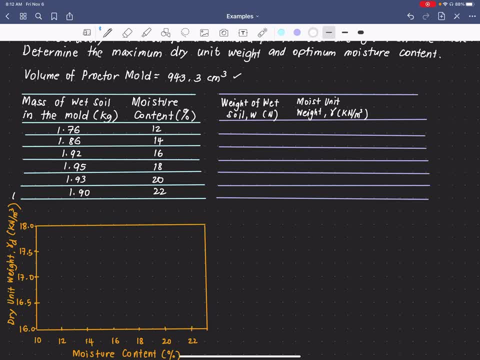 After calculating the moist unit weight, since we have the moisture content, we can get the dry unit weight, Or this is our gamma d, Also in kilonewton per cubic meter. So to solve for the wet unit weight- Sorry for the weight of wet soil. 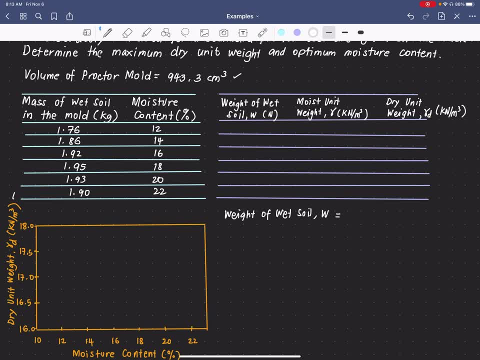 We simply multiply the mass, which is in kilogram, by 9.81.. So in doing this calculation, let us have one trial. Say W is equal to 1.76.. We have the first trial multiplied by 9.81.. 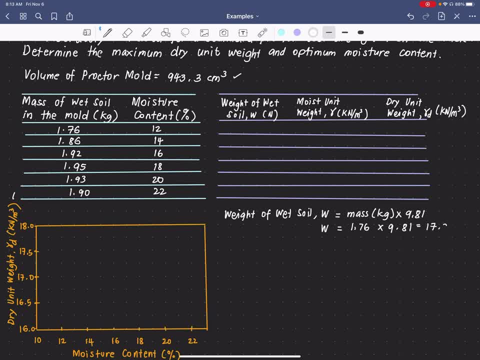 And this will give us 17.27.. So this is 17.27.. This is for the first trial, And if we will do the same process for all, the mass of wet soil will be getting the following values: 18.25.. 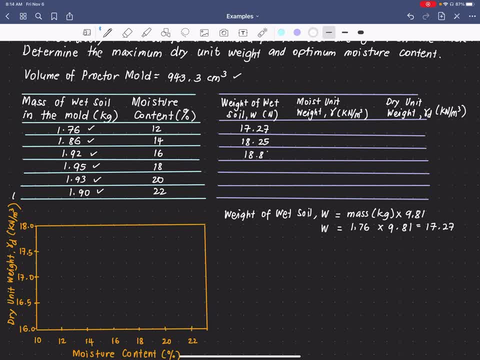 18.25., 18.84., 19.13., 18.93. And 18.64.. Notice that the weight is increasing at first 17. 18.25., 18.34., 19.95.. 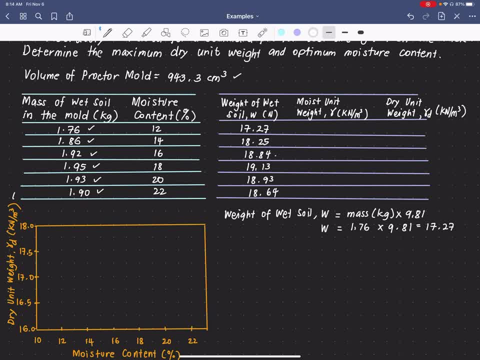 19.3.. But after some time the weight decreases: 18.93 and 18.64.. That's actually how we do it in the laboratory. We allow the increase of moisture content, while the mass of wet soil in the mold is increasing. 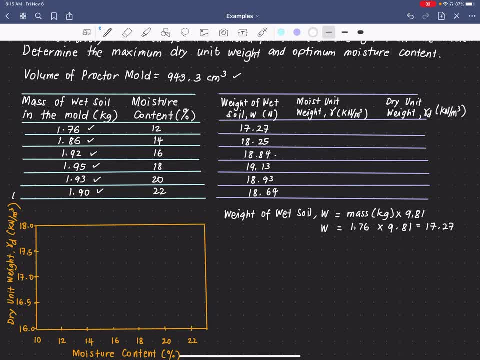 But after the time that it decreases we'll have like two trials for decreasing weight And then we will see. So I thought I don't have time for something, so let's go ahead and find something else. So we're going to go to this test. 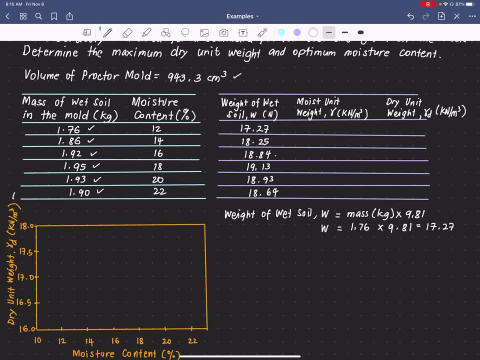 And then I'm going to try to stop the test because we can now come up the compaction curve. completely seemed already. So we can right now turn the motionaly map- type option And we can now calculate the mass of wet soil. 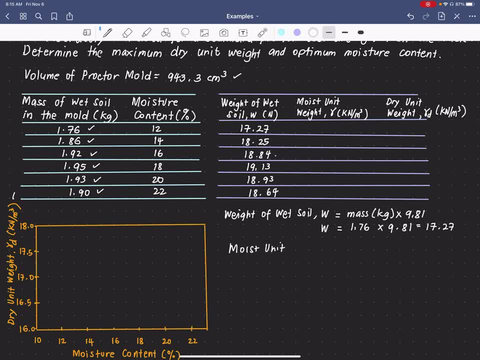 And so it will deal with the weight that comes from. must be those adds thehearted learning coming from what we've already done a few days ago. we can now ask the data, we can now draw the compaction curves, because with this data we can now draw the compaction curve. 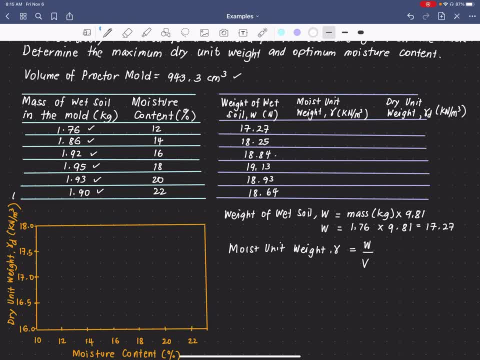 weight over the volume and it will get like: one sample you have: the weight here of this is 17.27, but this is in newton. to make it in kilonewton, because you want it in kilonewton, you have to multiply that by, or divide it by 1000. divided by the volume, the volume is 943.3. 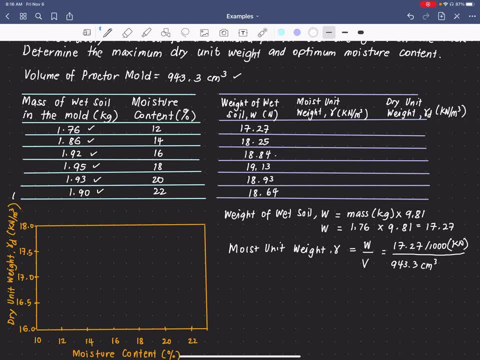 this is in centimeter cube. if you want this to convert to cubic meter we have to multiply this by times 10 to the negative 6, or 10 to the negative 6 to make it in cubic meter. so with this calculation we can get a value of the moist unit weight of. 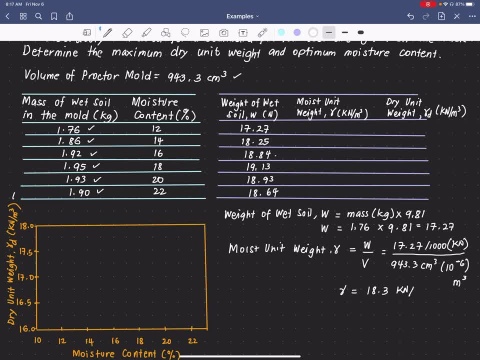 18.3. this is in kilonewton per cubic meter. so here we have 18.3 cubic meter and if we do the same process for all the trials, we'll get like 19.3 here, 20.0, 20.3, then it becomes 20.1 and then 19.8. so just do the same process. 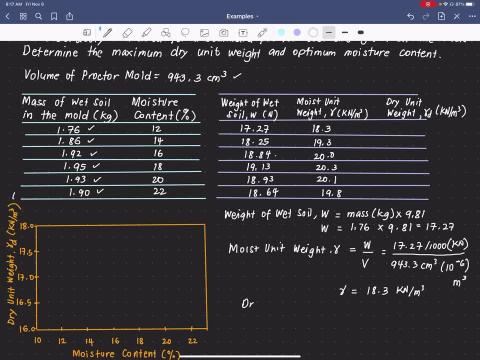 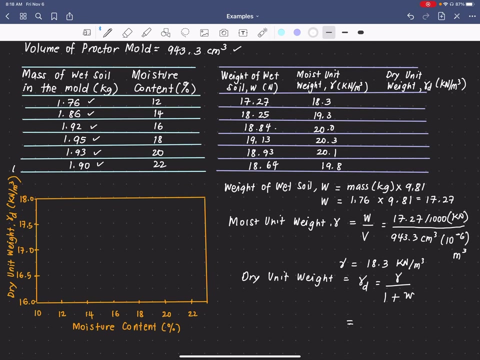 to get the value of the dry unit weight. so we have a relation that is: gamma dry is equal to the moist unit weight divided by 1 plus w. and let's have the first trials again. we have uh, gamma d equals 18.3 divided by 1 plus our unit weight is 12. this has to be divided by 100. 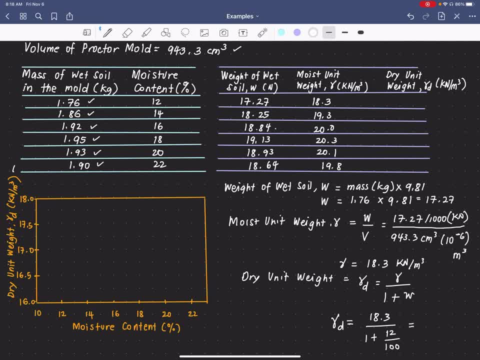 because this is in percentage and we can get the dry unit weight, which is equal to 16.34 kilonewton per cubic meter. so this becomes 16.34 and the next trial is 16.93. after doing the same process, 17.24. here we have 17.2. 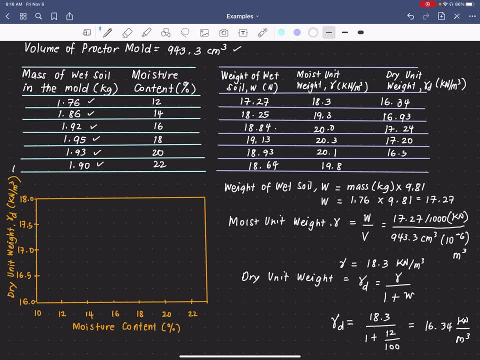 we have 16.5, 16.2 and 16.23. now, since we already have the values of the dry unit weight and the moisture content here and here, then we can just simply plot this data points here in our graph so that we can draw the compaction curve and subsequently determine the maximum. 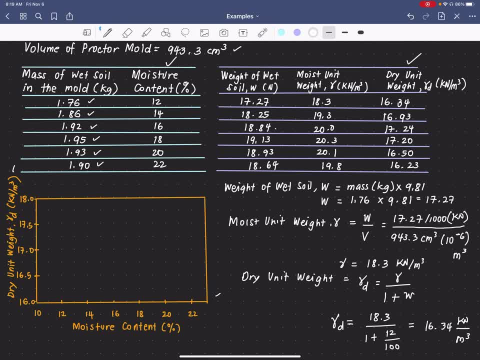 dry unit weight and the optimum moisture content. so for the first trial we have a moisture content of 12 and a dry unit weight of 16.34. so let us say this is our 12 and this is the 16.3, this is 16.5, 16.25. so let us say this is our first data point. 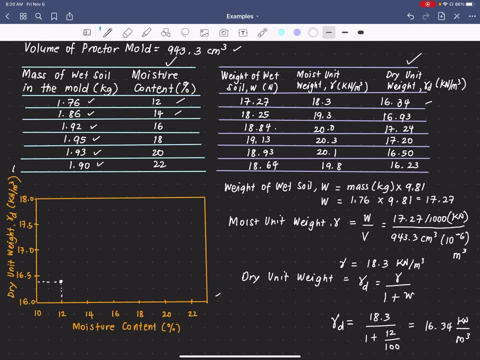 then the next moisture content is 14 and we have a dry unit weight of 16.93. so this is 14, and 16.9 is here, which is very close to still close. let's put, let's make it closer. there you go. so this is our second data point. then our third data point is 16 and 17.24. 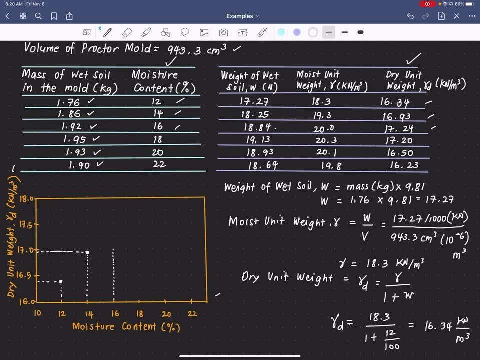 this is our 16, 17.24. so this is 17.25, so very close to 25, of course, and here's our third data point. then we have a moisture content of 18 and a dry knit weight of 7.2. so we have a dry knit weight of 7.2. 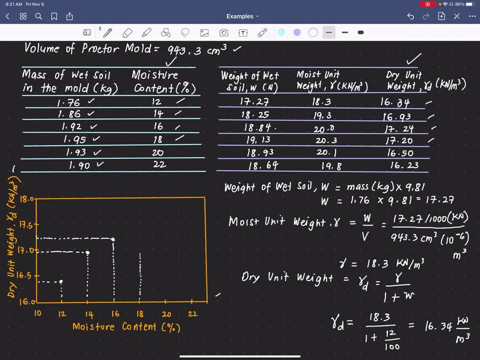 so we have a dry knit weight of 7.2. so since this is 7.2, that means the dry knit weight already decreases, start decreasing. so this is 25, 24 and we have 20. so that's just very close here. let's see, this is our fourth data, fourth data point, and we have 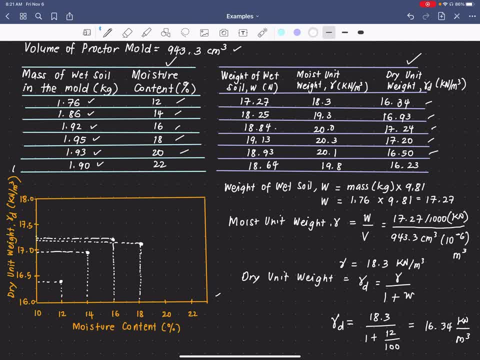 the fifth one, which has a moisture content of 20 and a dry unit weight of 16.5. there you go. we have 16.5. here's our 16.5. and here is our fifth data point. and we have 16.5. here's our 16.5. 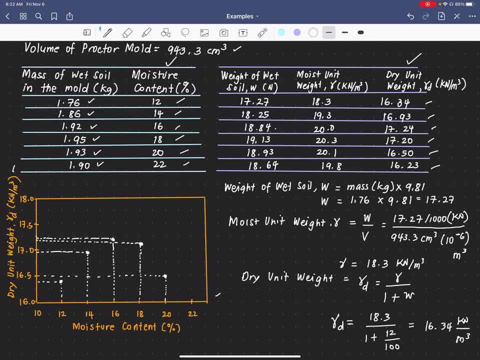 and here's our sixth data point. and we have 22 and 16.23. we have 22 and 16.23, let's say it's here and 16.23, let's say it's here. and here's our fourth data point. and here's our fourth data point. 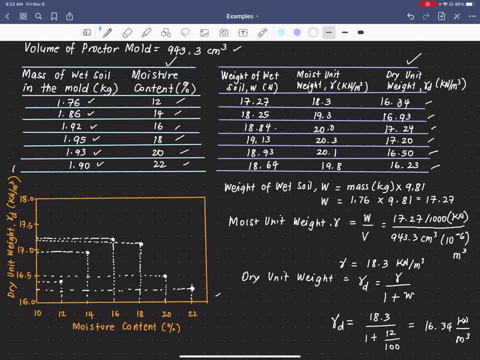 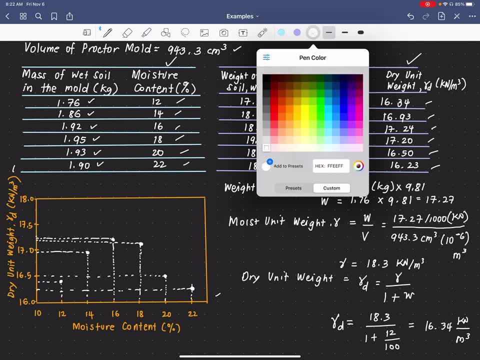 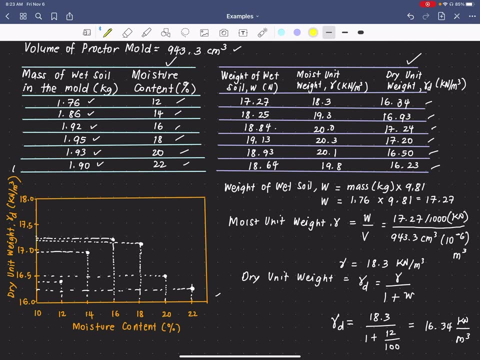 and here's our sixth data point, and here's our fifth data point. then the next thing to do is to draw a regression curve. then the next thing to do is to draw a regression curve, although it's quite difficult to do it, although it's quite difficult to do it here.